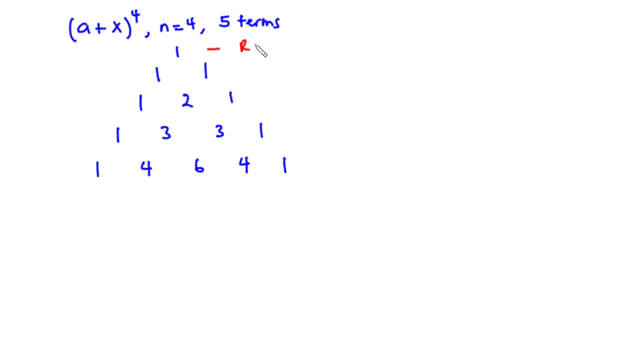 So the first one is rho zero. We have rho 1, rho 2, rho 3 and then rho 4.. So these are the coefficients of a binomial a plus x raised to the power 4.. Now we can as well use the method of combination to determine. 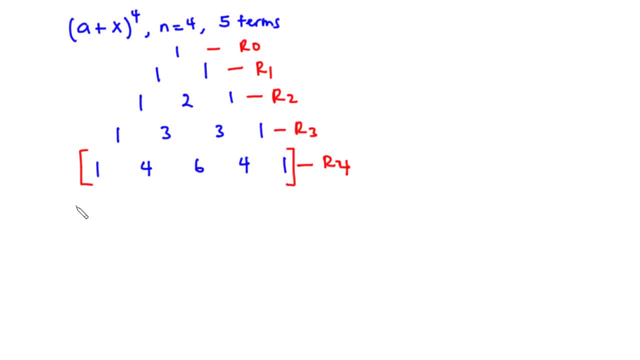 the coefficients of this binomial. So n combination r can sometimes be written as n r, this way vertically: And this is equal to n factorial over n minus r factorial times r factorial. So n combination r is equal to n factorial over n minus r factorial times r factorial. 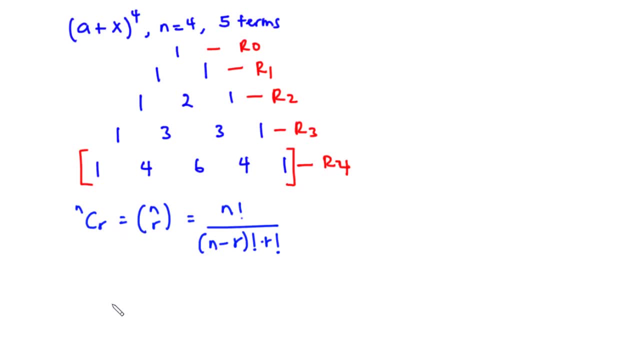 Now n combination r basically describes the number of ways of selecting r objects from n different objects, The number of ways of selecting r objects from n different objects. So back to the Pascal's triangle. this becomes 4 combination 0,, 4 combination 1,, 4 combination 2,. 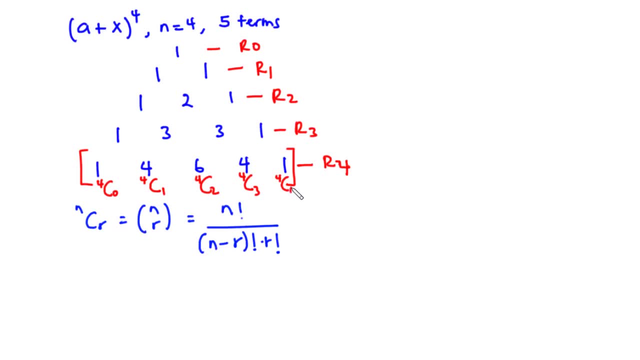 4 combination 3, and then 4 combination 4.. Now let's confirm our answer using the combination method. So let's say, if we are going to pick 4 combination 2,, we are going to pick 4 combination 2,. 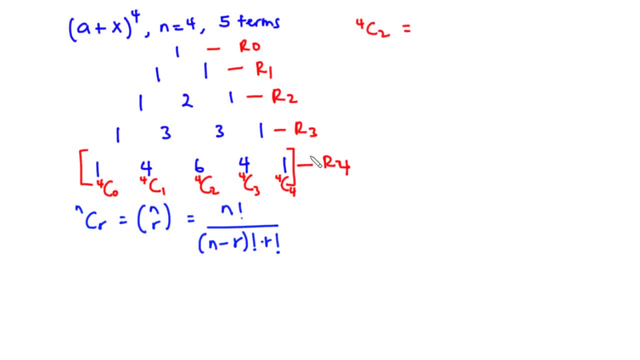 then 4 combination 2 is equal to 4 factorial over 4 minus 2 factorial times 2 factorial. You want to see if you are going to get 6.. Now 4 factorial is 4 times 3 times 2 times 1, divided by 4. 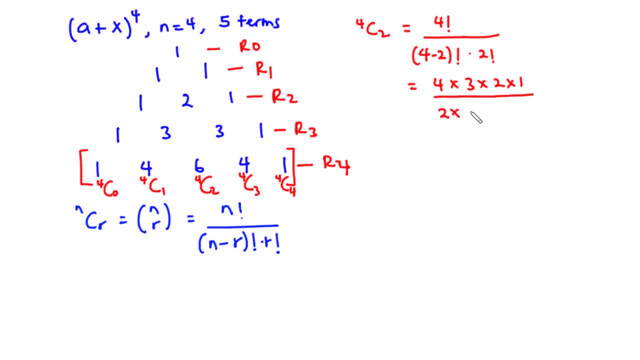 4 minus 2 is 2, so 2 factorial is 2 times 1, and then 2 factorial is also 2 times 1.. So this cancels out this. 2 goes into itself once, into 4 two times. 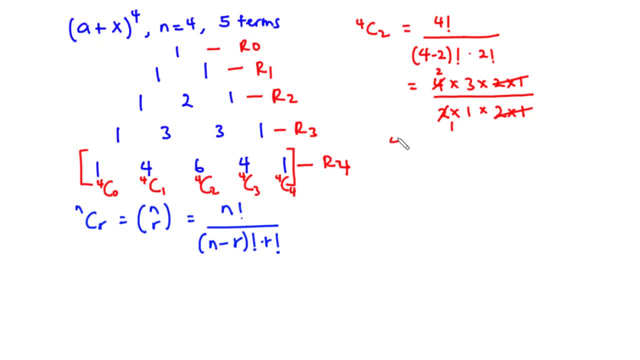 So we are left with 2 times 3, which is 6.. So 4 combination 2 is equal to 6.. So we can as well use the method of combination to determine the coefficient of a binomial expansion, without using the Pascal's triangle. 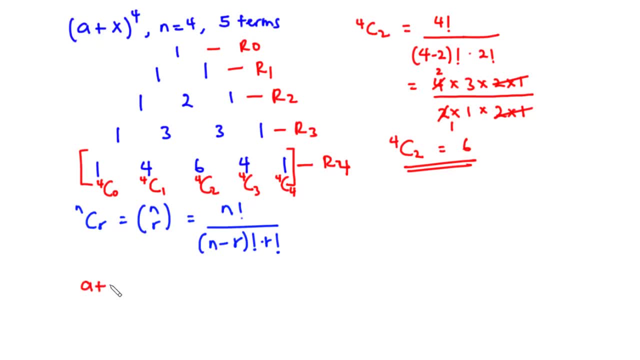 So the expansion of a plus x, raised to the power n, which is equal to a exponent n plus n times a exponent n minus 1 times x plus n times n minus 1, a exponent n minus 2 x squared over 2 factorial, and so on and so forth, can be written as: 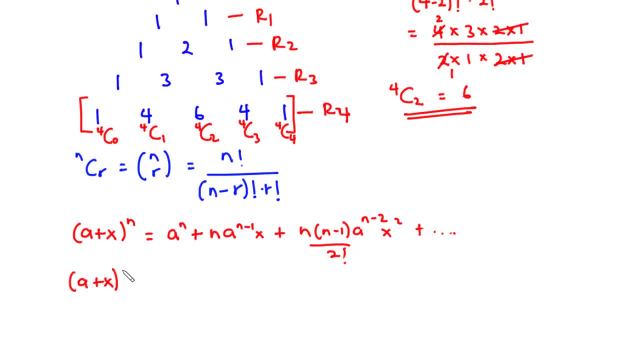 a plus x exponent n is equal to n combination 0 times a exponent n plus n combination 1 times a exponent n minus 1 x plus n combination 2, a exponent n minus 2 x squared, and so on and so forth. Note that n combination 0 is equal to 1, and then n combination n is also equal to 1.. 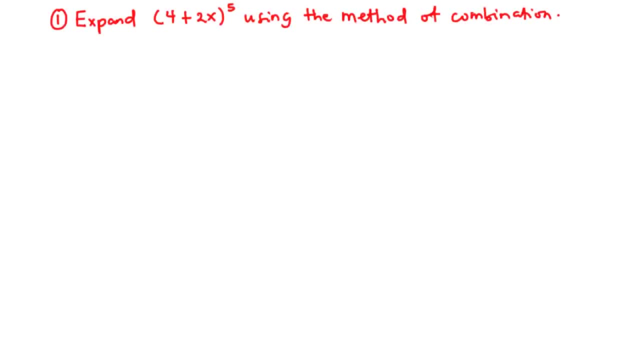 Now let's try some examples. So let's solve our first example, Example 1.. Expand the binomial 4 plus 2 x exponent. 5. Expand the binomial 4 plus 2 x exponent. 5. Using the method of combination. 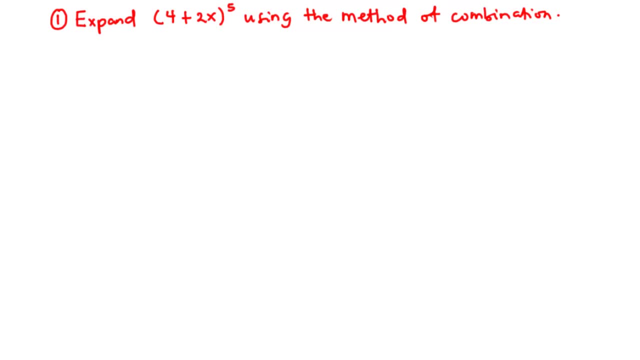 Expand 4 plus 2 x exponent 5.. Using the method of combination. So let's try this example together. So the binomial expansion of a plus x raised to the power n using the method of combination, is given by n combination 0 times a exponent: n plus n combination 1.. 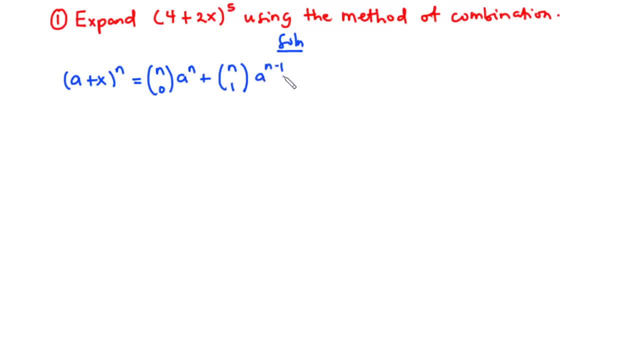 1 times a exponent n minus 1 times x plus n combination. 2 times a exponent n minus 2 x squared plus n combination: 3. A exponent n minus 3x cubed plus n combination. 4. A exponent n minus 4 x exponent 4.. 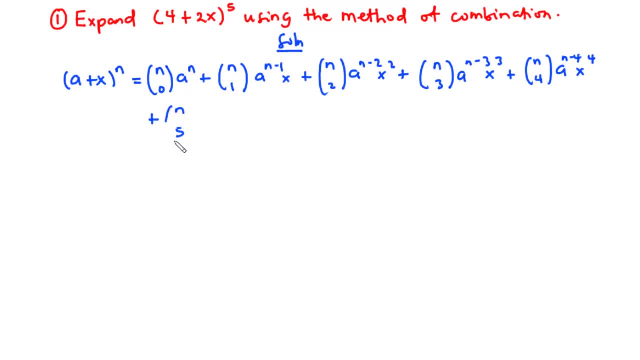 plus n combination 5, a exponent n minus 5, x exponent 5.. Now, because n is equal to 5, we are going to end at x exponent 5.. Now let's compare the binomials: a plus x raised to the power n. 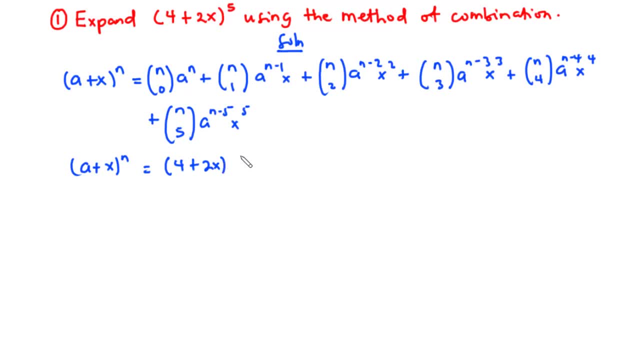 and then 4 plus 2x raised to the power 5.. So by comparing, a is equal to 4, x is equal to 2x and then n is equal to 5.. So let's find the expansion of 4 plus 2x exponent 5.. 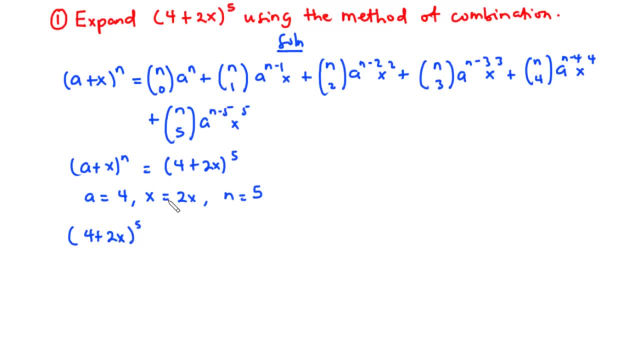 By this we are going to substitute the values of a, x and then n into this equation, So that's going to be 5.. Combination 0, we have a to be 4.. So 4 exponent 5 plus 5 combination 1 times 4 exponent 5 minus 1 is 4.. 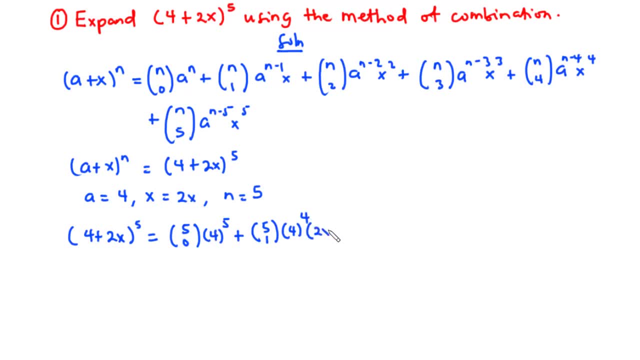 So 4 times x is 2x, So 2x plus 5 combination 2, 4- exponent 3, 2x exponent 2 plus 5 combination 3, 4- exponent 2, 2x exponent 3 plus 5 combination 4,. 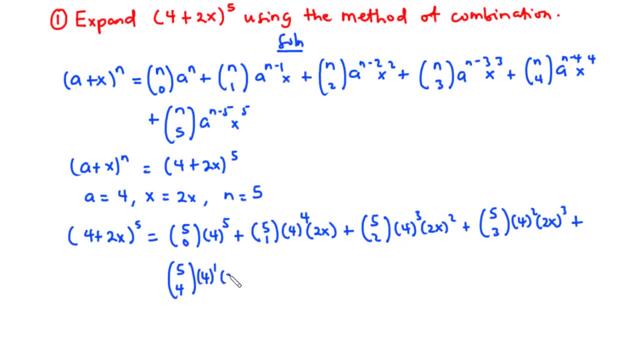 4 exponent 1, 2x exponent 4 plus 5. combination 5, 4 exponent 0 is 1.. So we leave that one out, and then we have 2x exponent 5.. So now let's simplify. 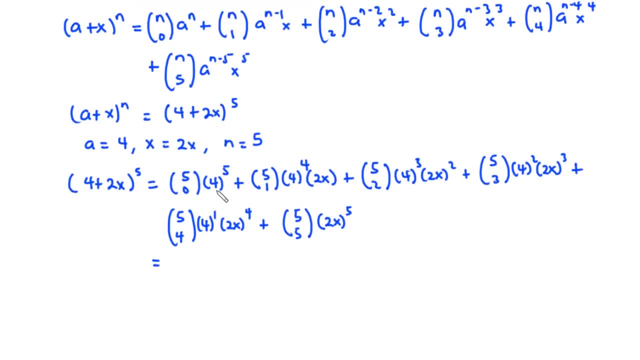 5 combination 0 is 1.. And then 1 times 4- exponent 5 gives 1024, plus 5 combination 1 is 5.. 4 exponent 4 times 2 gives 512,. times x plus 5 combination 2 is 10.. 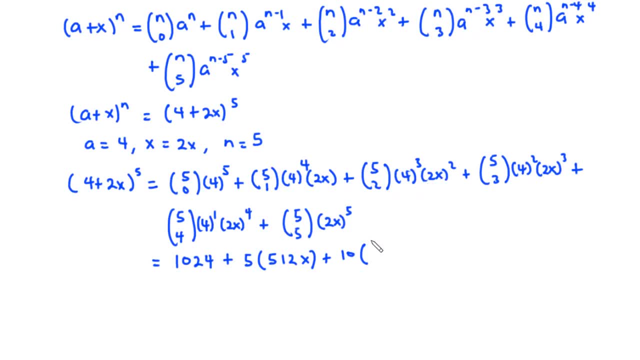 4 cube times 2 square gives 256.. And then x square plus 5, combination 3 is 10, times 4 square, times 2 cube gives 128.. So 128x cube plus 5, 5, combination 4 is 5.. 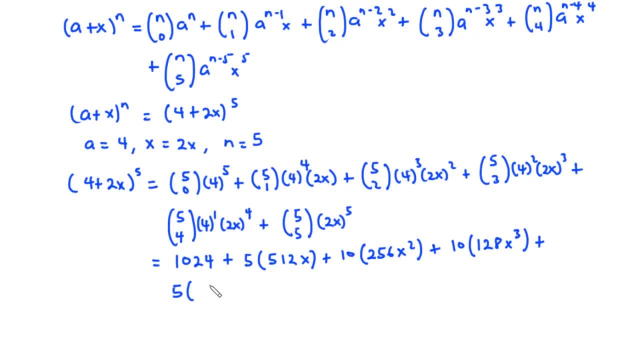 4 exponent. 1 times 2 exponent 4 gives 64.. So 64x exponent 4 plus 5, combination 5 is 1.. Now 1 times 2 exponent 5 is 32.. So 32x exponent 5.. 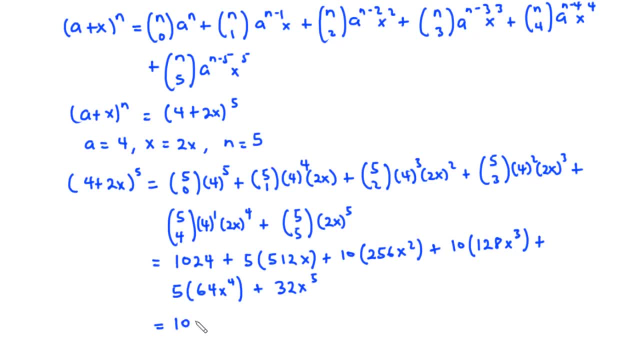 So let's simplify further. We have 1024 plus 2560.. So 2560x plus 10 times 256 becomes 2560, and then x square plus 10 times 128 gives 1280x. cube plus 5 times 64 is 320.. 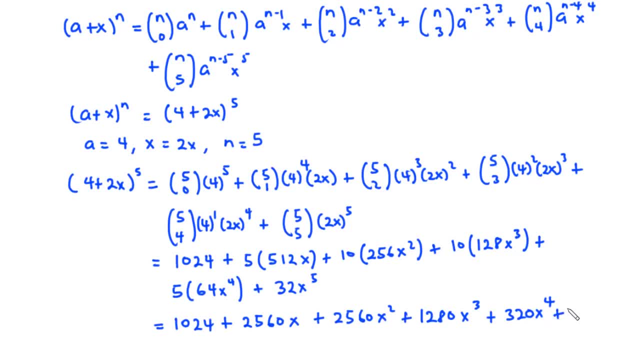 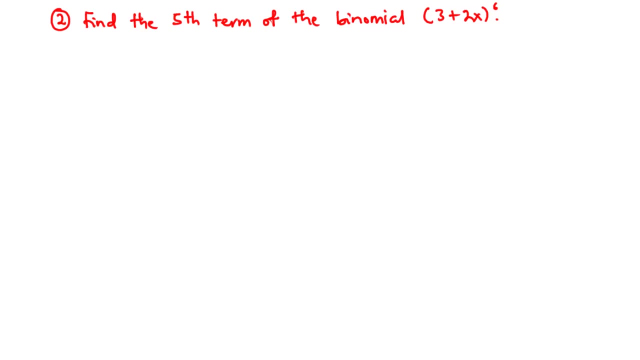 So x, exponent 4 plus 32x exponent 4.. So this is the binomial expansion of 4 plus 2x exponent 5, using the method of combination. Now let's solve the second example. So what if we just want to find only one term of a particular binomial expansion? 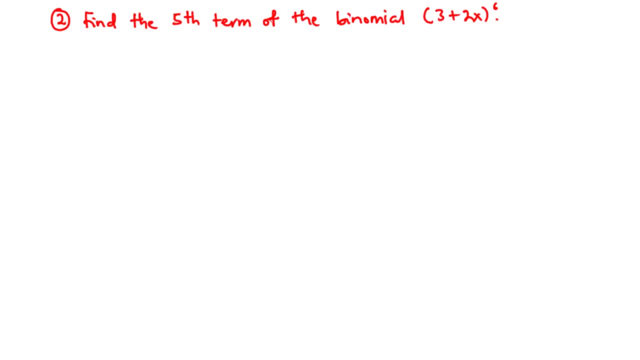 Now that leads us to our second example. Find the fifth term of the binomial 3 plus 2x, exponent 6.. So we are just going to find the fifth term of this expansion Now. we don't need to write down all the terms of this binomial expansion. 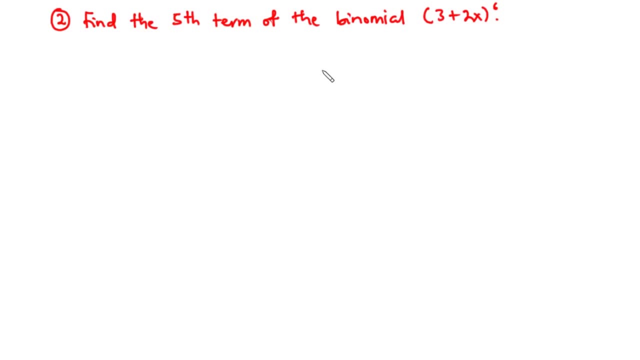 so that we pick out the fifth term. However, we can use the method of combination to find the fifth term of the binomial, without necessarily expanding to find all the terms. So that is what we are going to do. So let's compare the binomial a plus x. 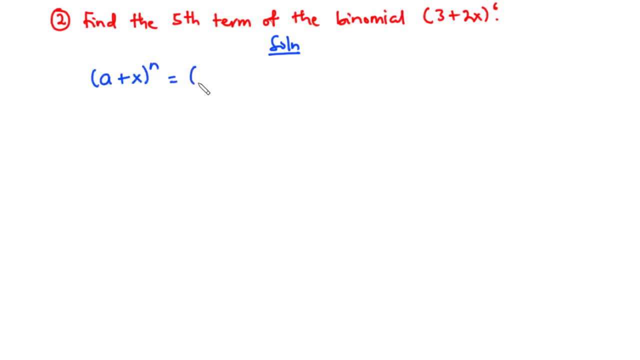 raised to the power x Or n to the binomial given in the question, 3 plus 2x, exponent 6.. So by comparing, we have a to be 3, x to be 2x and then n to be 6.. 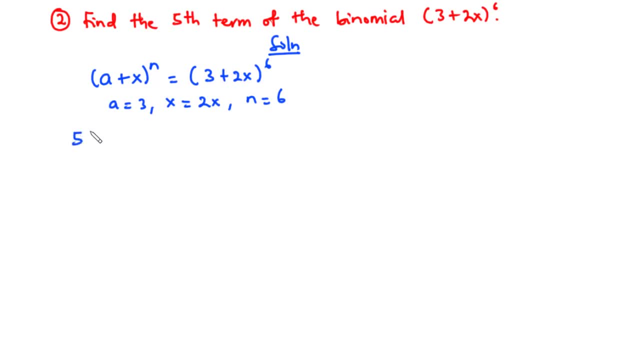 Ok, So the fifth term of the binomial expansion of 3 plus 2x exponent 6.. is going to be the fifth term of the binomial expansion of 3 plus 2x exponent 6.. never mind, exponent 6 can be found by using the formula n combination r times a. 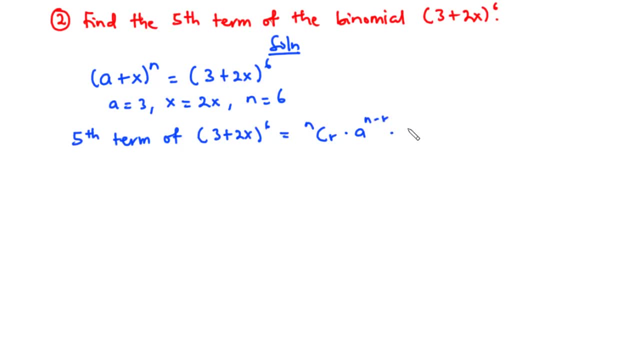 exponent n minus r times x exponent r. Now we have the values of a, x and then n, So we can substitute those values into this formula to find the fifth term of the binomial 3 plus 2x, exponent 6.. So we have n to be 6.. So 6 combination. 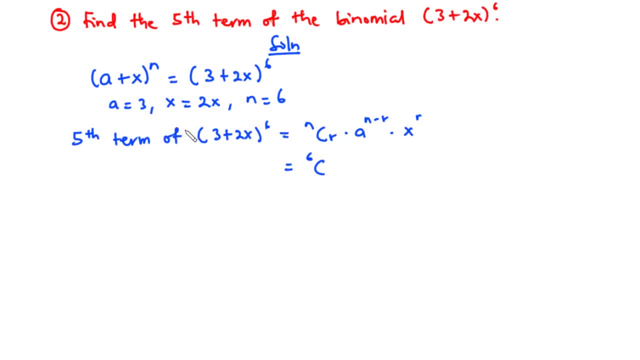 Now to find r. we are going to subtract 1 from 5 because we are going to find the fifth term is going to be 5 minus 1, which is 4.. So 6 combination 4 times we have a to be 3.. So 3 exponent: 6 minus 4, which is 2.. 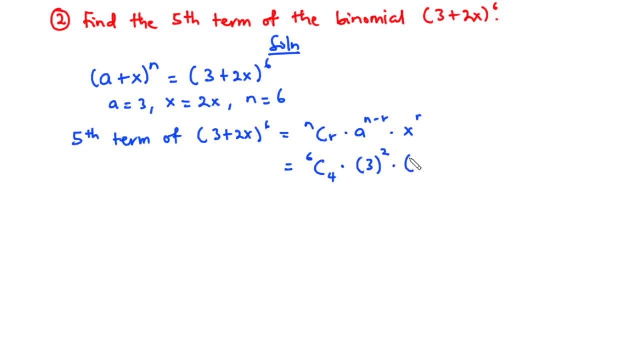 Times x is 2x, exponent r, which is 4.. Now let's continue. 6 combination 4 is the same as 6 factorial over 6 minus 4 factorial times 4 factorial 3, squared is 9.. So times 9.. 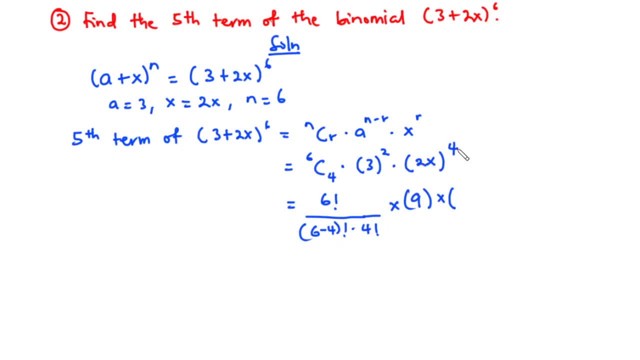 Times 2, exponent 4 is 16.. So 16x exponent 4.. So let's simplify further: 6 factorial is 6 times 5 times 4 factorial. Divided by 6 minus 4 factorial is 2 factorial. 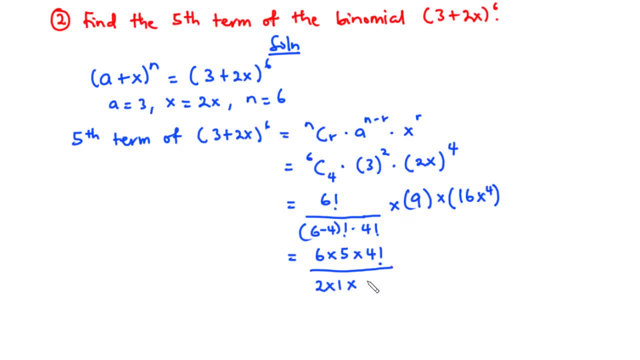 So that is 2 times 1 times 4 factorial Times 9 times 16x exponent. 4 gives 144x exponent 4.. 4 factorial cancels out 4 factorial 2 goes into itself once into 6, three times. 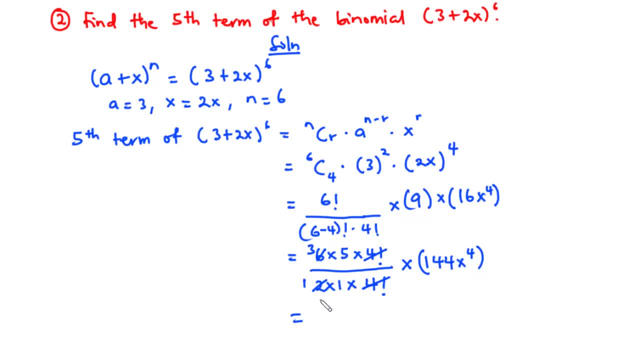 So we are left with 3 times 5 divided by 1, which is 15.. So 15 times 144x exponent 4.. 15 times 144 gives 2160x exponent 4.. So this is the fifth term of the binomial 3 plus 2x exponent 6.. 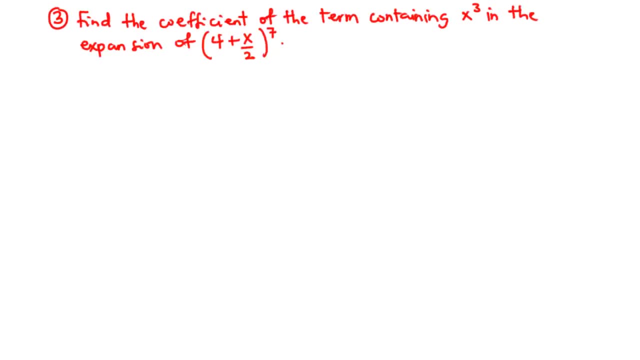 Now let's solve the next question. So to example 3.. Find the coefficient of the term containing x cube in the expansion of 4 plus x over 2, raised to the power 7.. Now the term containing x cube is the fourth term. 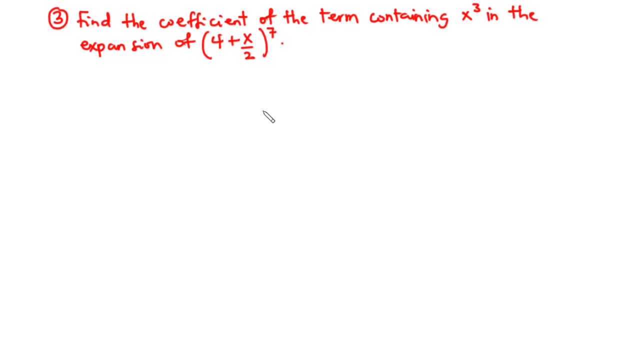 So, basically, we are going to find the fourth term of the expansion of 4 plus x over 2 raised to the power 7.. So, like we did in the previous example, Let's compare the binomials: a plus x raised to the power n equals 4 plus x over 2 raised to the power 7.. 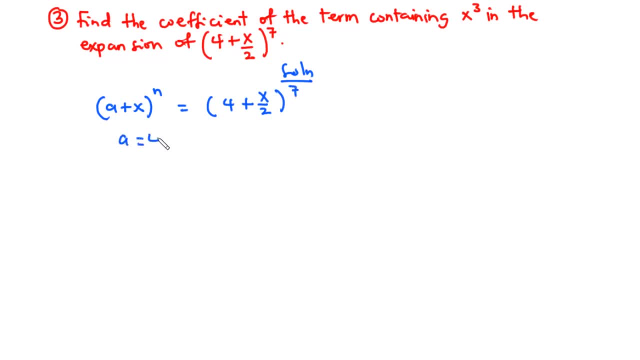 So, by comparing, we have a to be 4.. We have x to be x over 2.. And then we have n to be 7.. Okay, Now the fourth term Of the binomial expansion of 4 plus x over 2 exponent 7 is equal to n combination r times a. exponent n minus r times x exponent r. 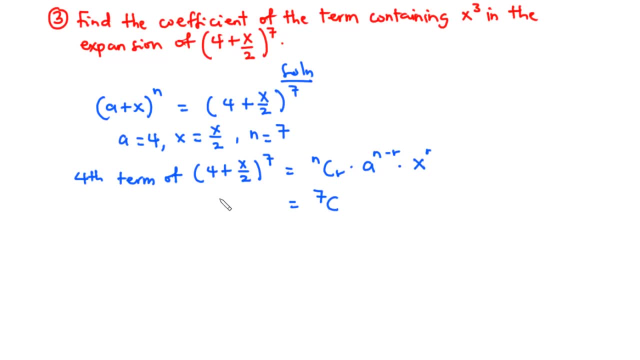 We have n to be 7.. So 7 combination, Because we are going to find the fourth term. Then it's 4 minus 1, which is 3 times a is 4.. So 7 minus 3 is 4.. 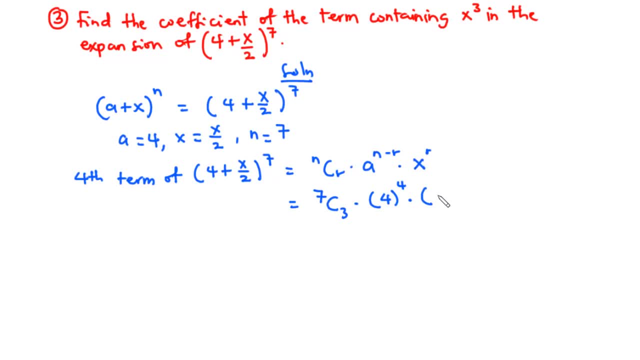 So exponent 4 times x over 2, exponent 3.. 7 combination 3 is 7 factorial over 7 minus 3 factorial times 3 factorial 4 cube gives 255.. 256 times this becomes x cube over 8.. 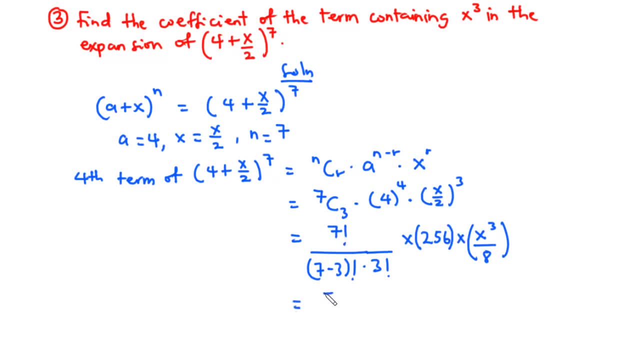 So let's simplify: 7 factorial becomes 7 times 6 times 5 times 4. factorial over 7 minus 3 is 4.. So we have 4 factorial Times 3 factorial is 6.. So times 6..